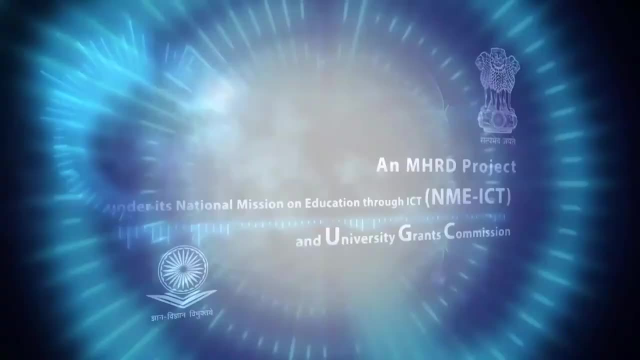 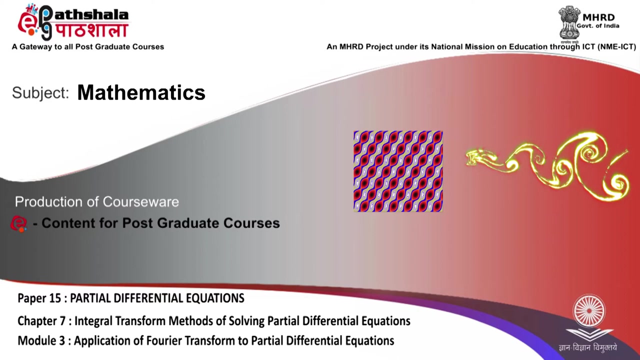 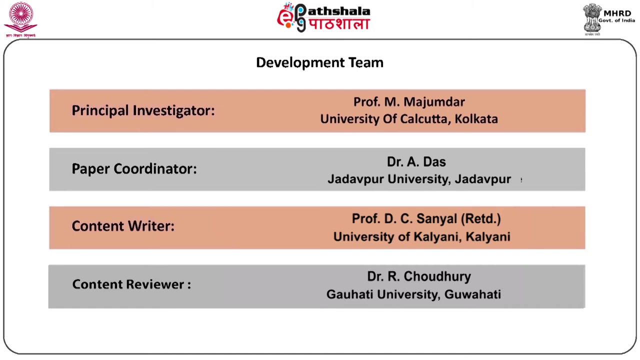 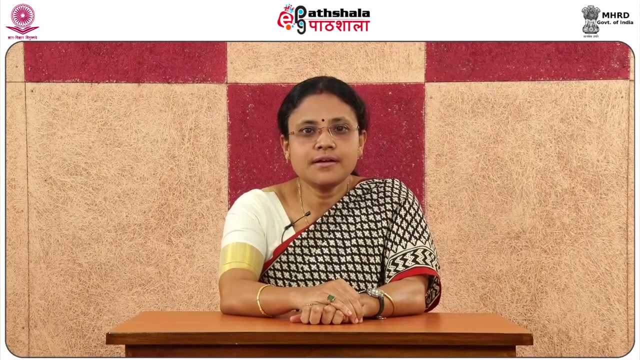 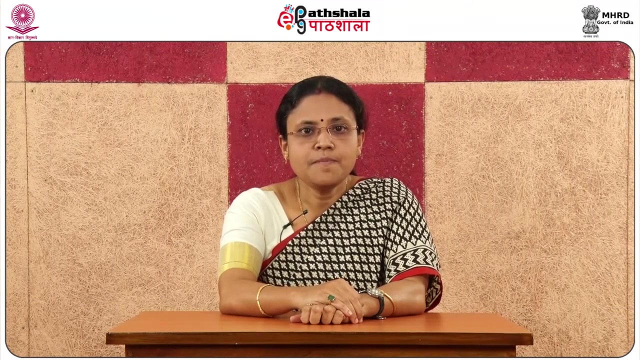 Now I am going to start module 3 of chapter 7.. In this module I want to mention that Fourier transform is a general transformation. Many other transformation, like Laplace transformation, Malin transformation, Henkel transformation, can be defined in terms of complex Fourier transformation. 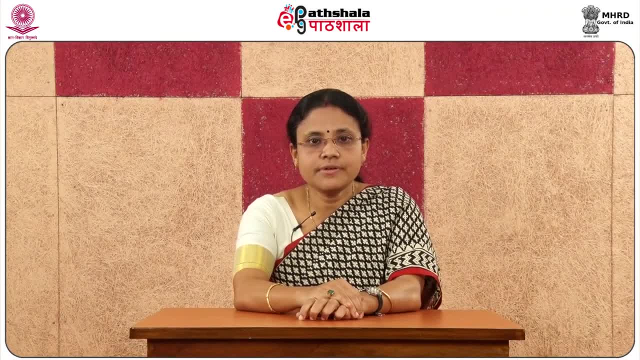 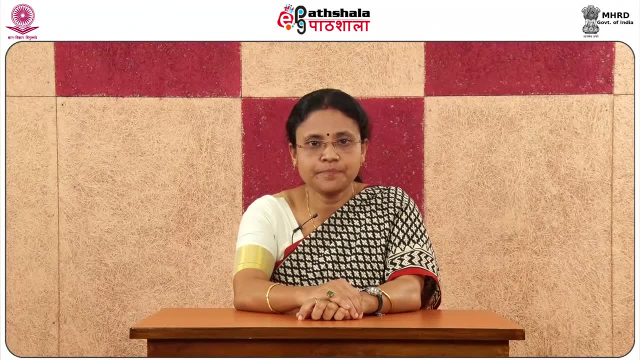 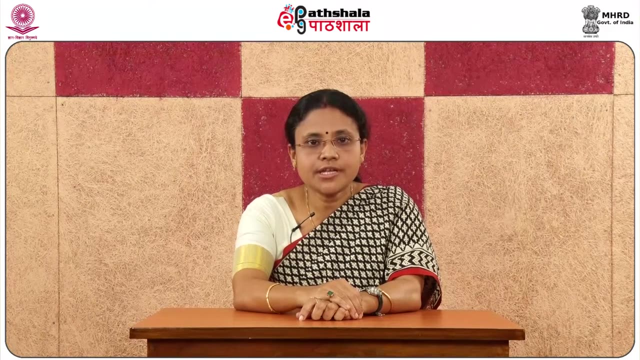 Therefore it is relevant to discuss about the application of Fourier transform to partial differential equation. In this module we shall solve the Laplace equation, heat equation and wave equation using Fourier transformation method. Now we are going to slideshow. First we shall start with Laplace equation. 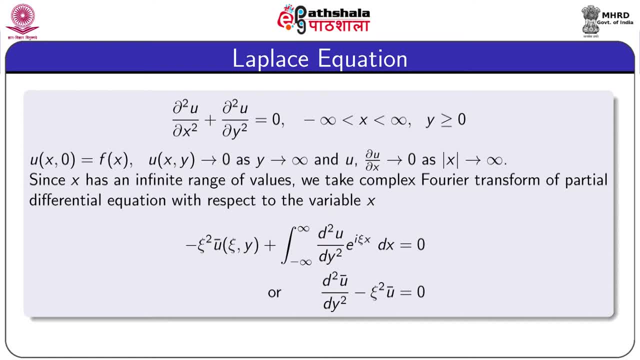 The Laplace equation in Cartesian coordinate system is given by del 2? u del t square plus del 2? u del y square equals to 0. Here we have considered infinite range for x and y is greater equals to 0.. We have also the initial condition for u: u at t equals to 0 is equal. 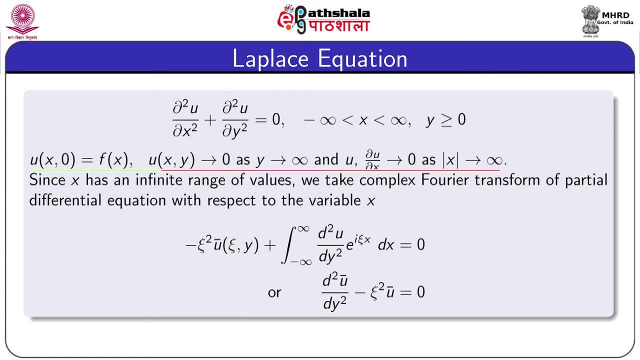 to f x. we also have u x. y tends to 0 as y tends to infinity. We have u del u del x. both quantity tends to 0 as mod x tends to infinity. Since x has infinite range of values, we take complex Fourier transform of the given equation with respect to variable x, So we multiply. 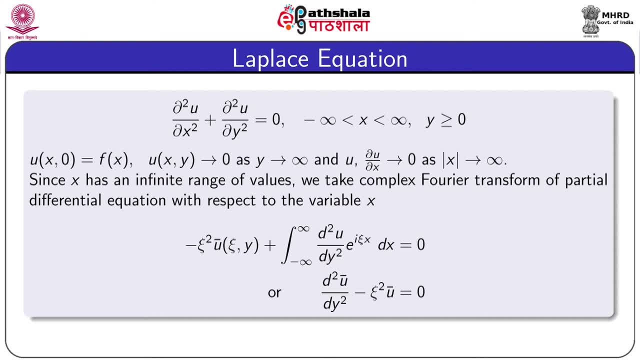 the Laplace equation with e to the power i xi, x, and then integrate over x from minus infinity to plus infinity. The first term gives minus xi square u bar xi, y and the second term is Plus integration. minus infinity to plus infinity, d to u, d, y square e to the power i, xi, x, d. 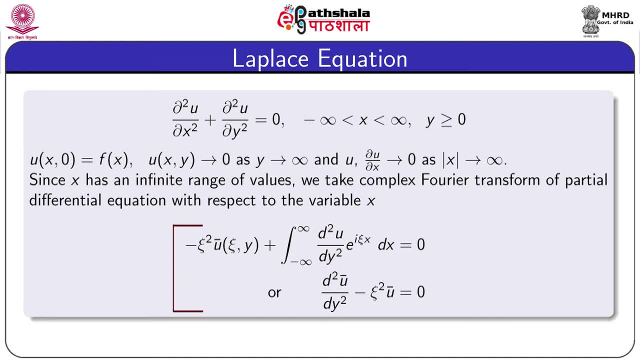 x equals to 0. Here xi is the transformed variable and the dependent variable, or u, is transformed to the function u bar. So u bar is now function of xi and y, if you look at the expression which is given by the integration in this integral. 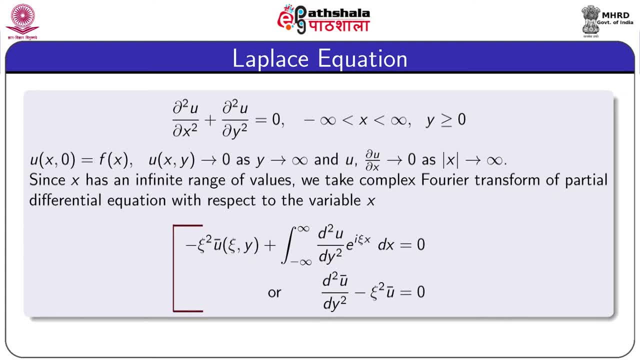 if we interchange the differential and integral operator, then it gives d to d, y square of integration. minus infinity to plus infinity, u into e to the power, i, xi, x, d, x. So that is nothing but u bar. So the second term in the expression gives minus infinity to. 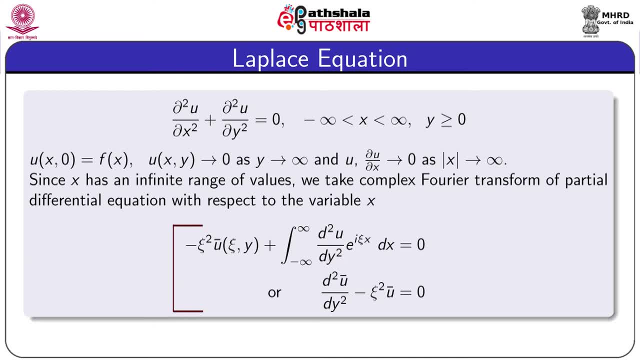 i, xi, x, d q. Record expression is d to u bar d y square and the first term is minus xi. square. u bar equals to J. undefended equation with respect to infinity: u index operation: 2 times any constant: z, Fuel 800, сv, e into 3,. minimum question: 2 times dynasty. u stress 1 by 3.. 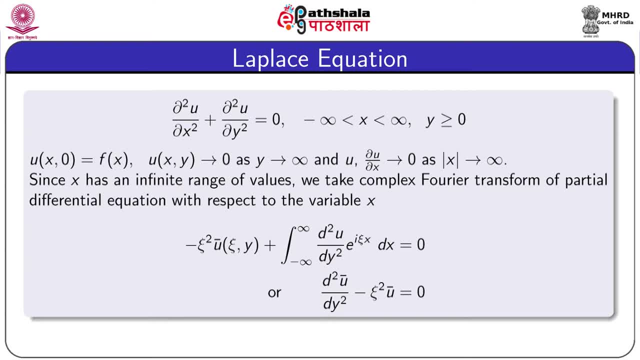 Now this is the resultant equation. This is an ordinary second order differential equation in u bar. The solution of this equation can be written easily. It is a into e to the power z, comma 1.. So the initial equation. you are interested. 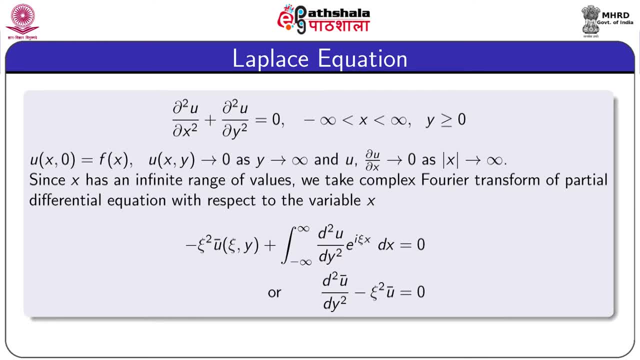 most acute equipment is here red, and then replaced it with a, and we do not need the new equation, because if we check the equation like this again, this polynomial equation is used like a constant equation. therefore, this particular name, productivity minus infinity, u, and then this polynomial Sebastian, f, z, s, e, into the power i, xi, xx, and then, despite this, we do not need the ум filing. 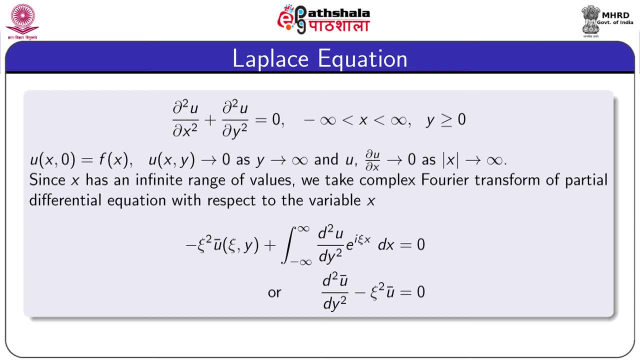 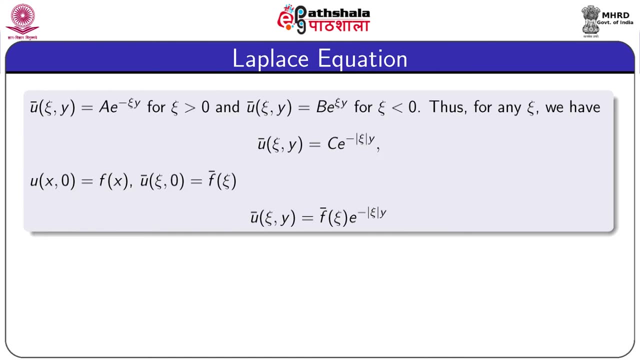 into y plus b into e, to the power minus xi into y, where a and b are arbitrary constants. Now to get the bounded solution, u bar should have the functional form: a into e to the power minus xi into y for xi greater than 0, and u bar equals to b into e. to the power xi- y. 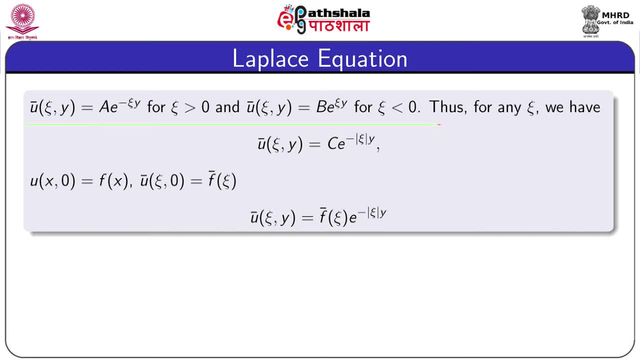 for xi less than 0. Thus for any xi we can write the solution in the form: u bar is equal to c into e, to the power minus mod xi into y. Now to find the value of c We need to apply the initial condition. The initial condition is given: u x 0 is equal. 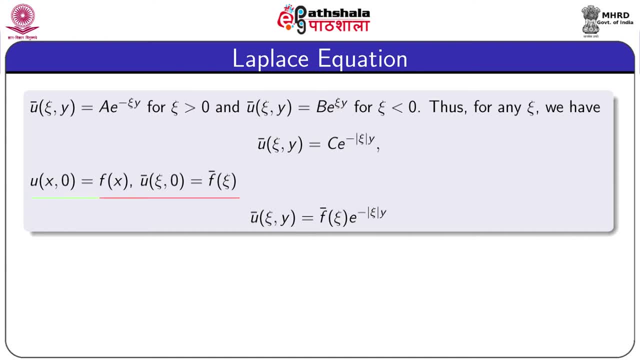 to f x. Now, if we apply the Fourier transform of this equation that gives u bar xi 0 is equal to some function: f bar xi. Now, if we use this condition, Now, if we use this condition, Now, if we use this condition, 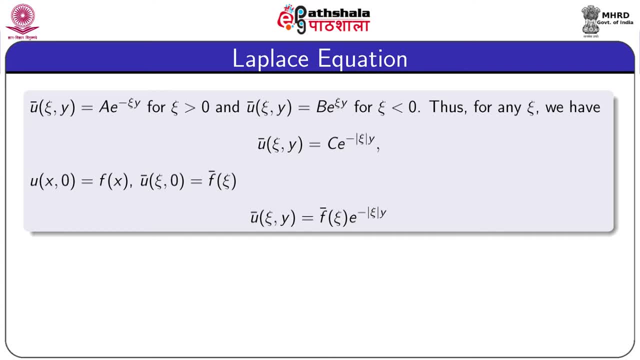 To the solution: u bar equals to c, e to the power minus mod xi, y. this gives the value of c is equals to f bar xi. Now, substituting the value of c in the general solution, our required solution, u bar, which is function of xi and y, is equal to f bar xi into e to 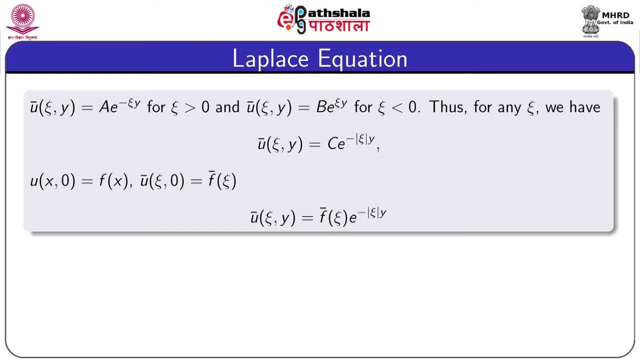 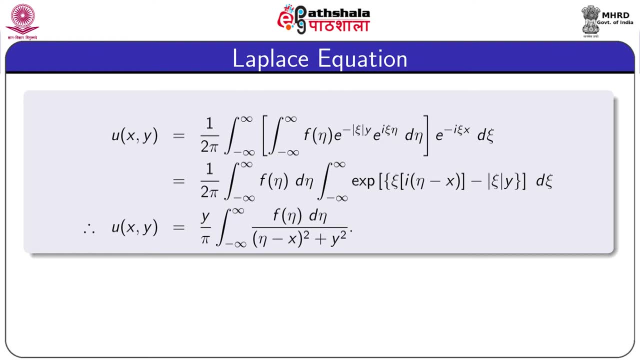 the power minus mod xi into y, And this is due to the Tao, to the value of phi y. that means v bar Banks out in the form ofista. Now we have to find u as function of x and y. That means from this solution: 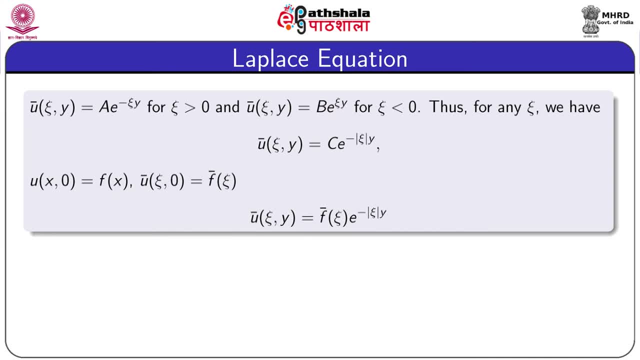 in the expression for u bar we need to apply inverse Fourier transform to find u as function of x and y. Now to obtain u as function of x and y which is given in the classical equation u bar inside 多 enough from this solution we apply inverse Fourier transform of u bar入 to � component 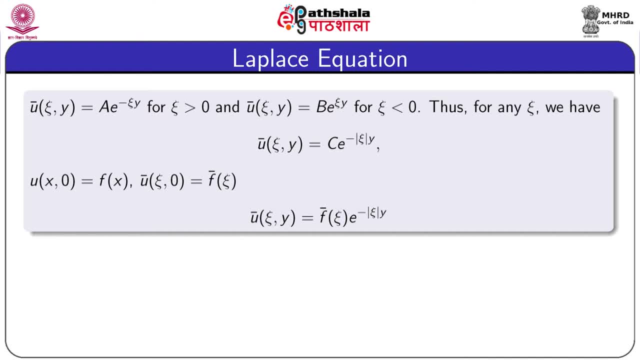 we have to apply inverse Fourier transform to find u as function of x and y. Now to obtain u as function of faki Shu AT. in the classical equation we name a new term, u bar as function of x and y. Therefor u bar will be zero for all xi y minus p d by tau. 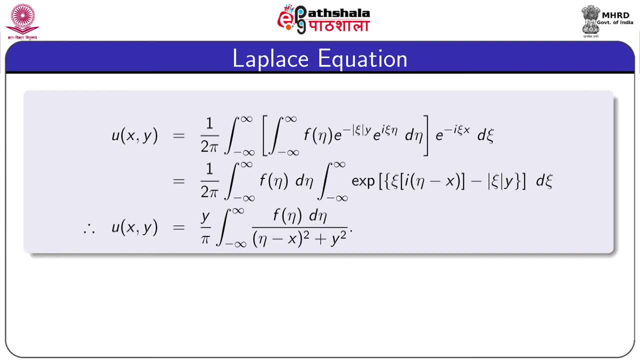 equal to f docrili, And y equals to 0. And y equals to b over xi function of x and y. we need to apply inverse Laplace transform of u bar. So the formula is written here: u is equal to 1 by 2 pi integration minus infinity to plus infinity, e to the power. 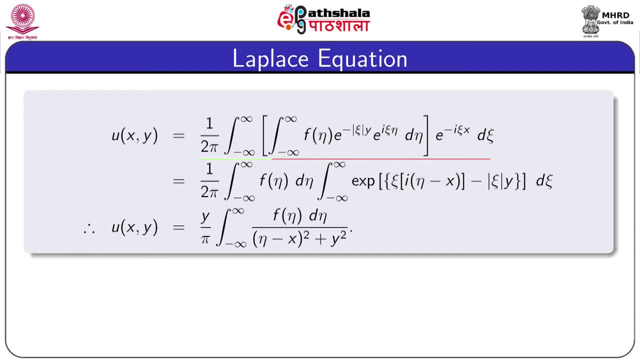 minus i xi x into f bar xi, And we have also substituted the value of f bar xi, which is written here, minus infinity to plus infinity, f eta e to the power, minus xi y e to the power i xi, eta, d eta this. So in the next line this is equals to 1 by 2 pi minus infinity to plus infinity, f eta. 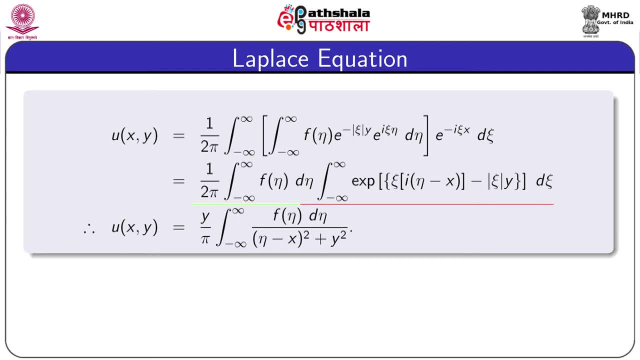 d eta into integration. minus infinity to plus infinity, e to the power, xi into i eta, minus x, minus mod, xi into y d xi. In the second line we interchange the order of integration. So we are processed. Now we can evaluate the seven second integral and the value of the. 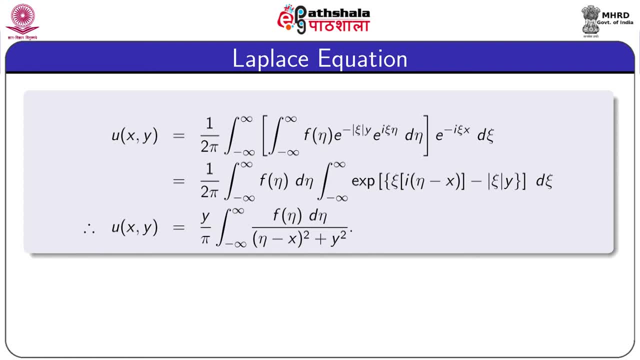 second integral is 1 divided by eta minus x hole square plus y square. Therefore our required solution: u function of x and y is equal to y by pi integration minus infinity to plus infinity, f, eta, d, eta by eta minus x hole square plus y square. So we can evaluate. 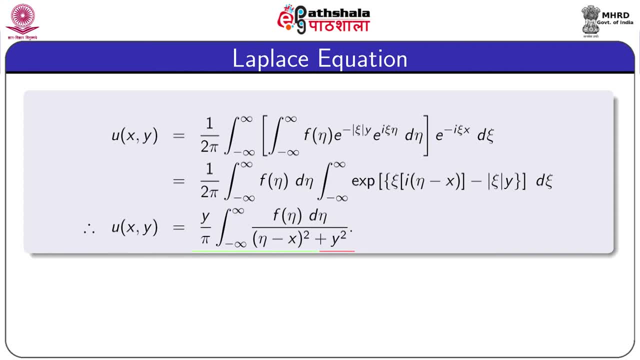 theiary of this second integral, which would be 1 by 2 pi dar e to the power 175.. So we get nowadays the recorded solution. you have to lying down the total express right value phi of psi or psi e to the power of phi, where pi equals phi to the power, into pi, into Cats. 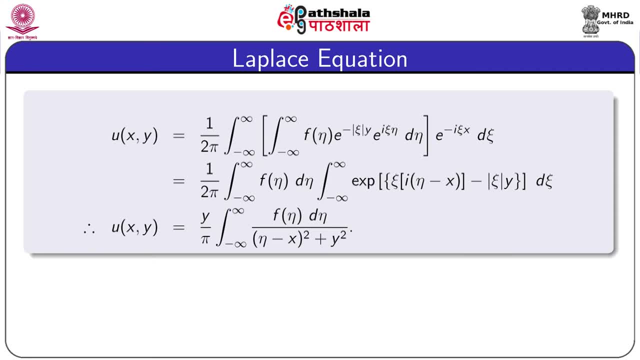 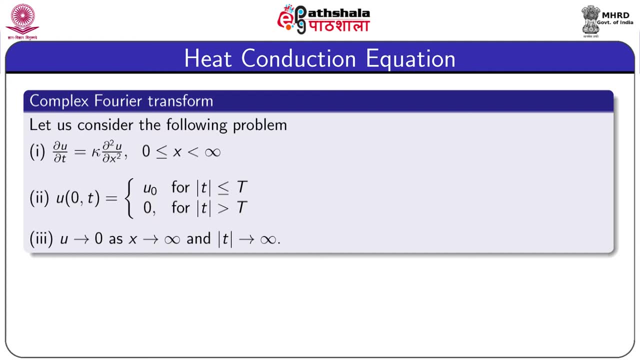 this will remain with the term psi. But now let us look at the same problem. solve for the second as y square. Now we shall consider heat conduction equation and we shall apply complex Fourier transform to find solution of this equation. So the 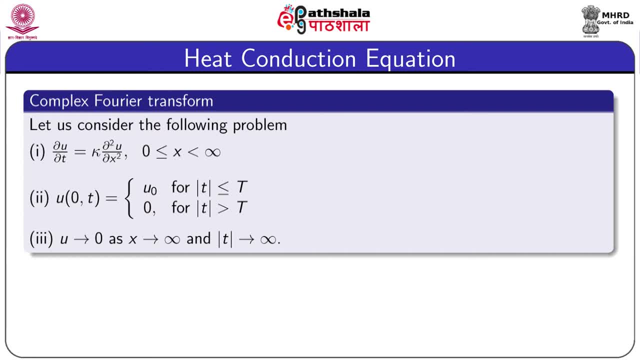 given equation is the heat equation, one dimensional heat equation in Cartesian coordinate system, which is given by equation: one del u del t equals to kappa del t? u del x square, where x lies between 0 to infinity, and this equation is satisfied with the given condition. This: